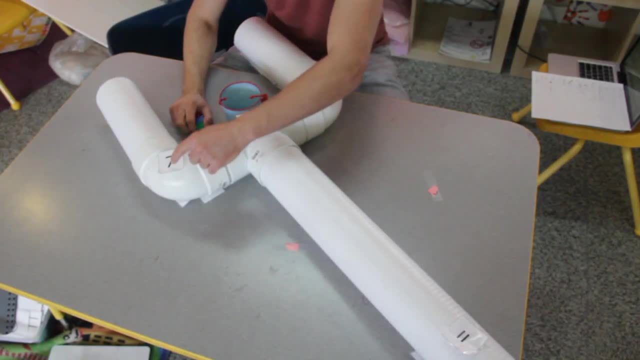 you can make this with any kind of piping and you have seven on this end, and if you have eight on this end and you have one kid, put seven down this and of course you want to make the sound effects. It's an adding machine after all, Or you could have the kids. 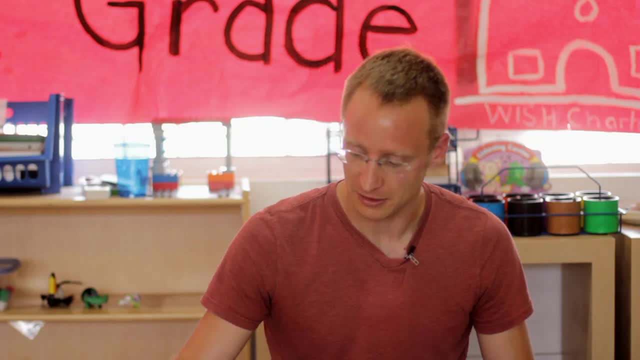 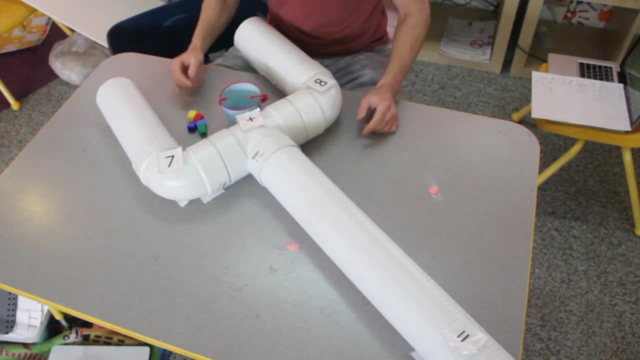 what kind of sound effect do you want to make when you put seven in the adding machine And there's seven on this side and there's eight on this side and they come together and equal how many? And then you pick up the adding machine off the ground and you look. 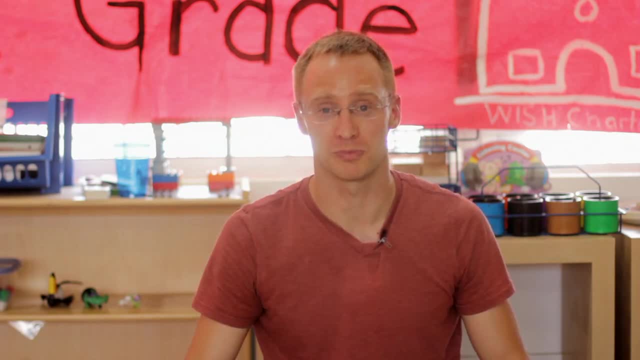 oh, let's count them kids. and then you do your one-to-one correspondence up to 15.. What kids got to see then was that they were able to do a lot of things. They were able to do a lot of things. So the idea there is: you had one group on one side and one group on 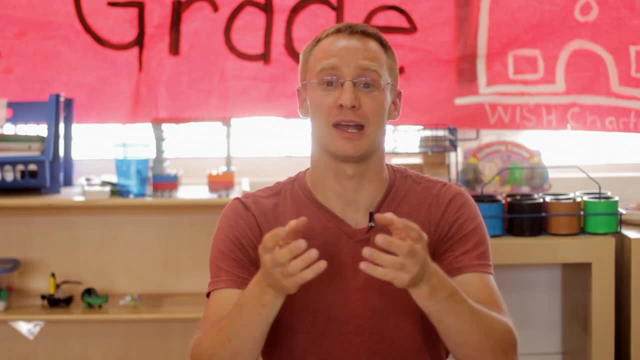 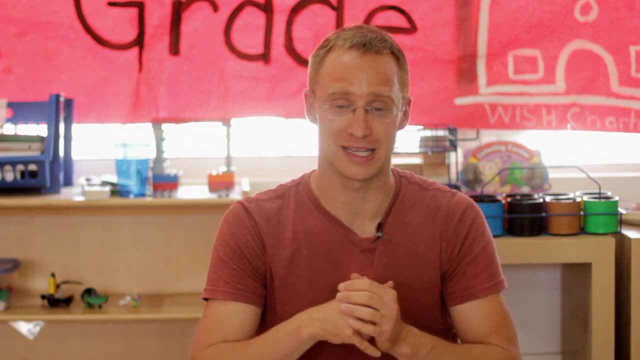 the other, on different sides of the adding machine, and they came together to form a whole new group. So that concept is actually visualized and acted out and carried out and touched with the adding machine- Another one you can do that's going to help kids understand. 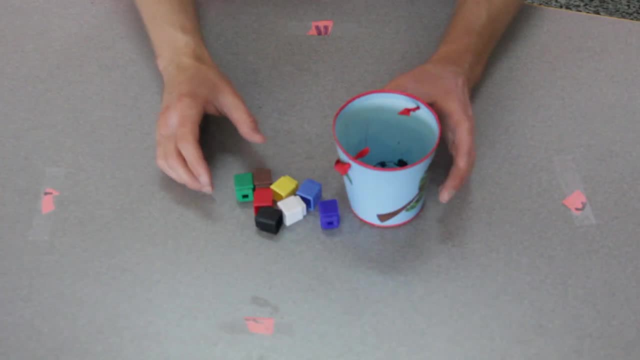 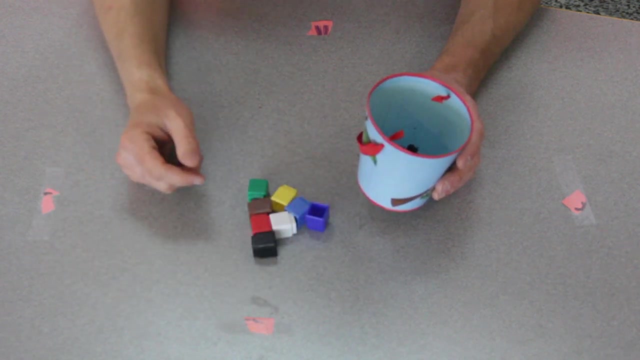 the concept of adding is Fill and Dump. With Fill and Dump, you give every kid a cup and every kid a set of objects. You'll need a lot of them, so make sure you have at least 50, or whatever class that's going to be. 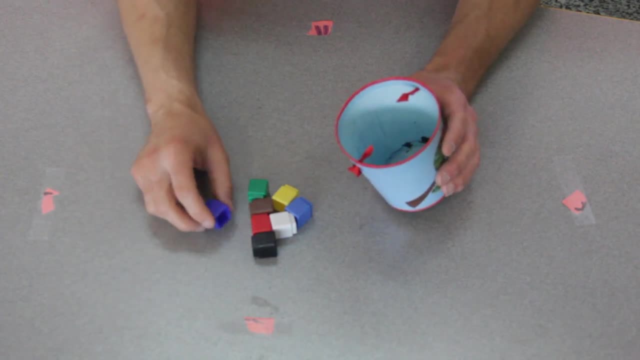 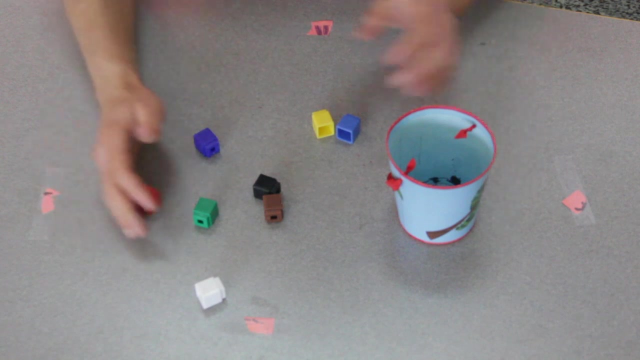 Because every kid's going to get from 8 to 10 cubes. And then you put it in the cubes. You say: kids, listen to me and follow these directions, Put in one and two more and three more. Dump How many all together. And then the kids have to count up how many they. 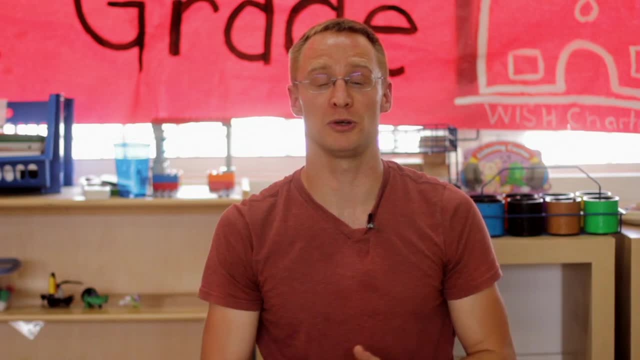 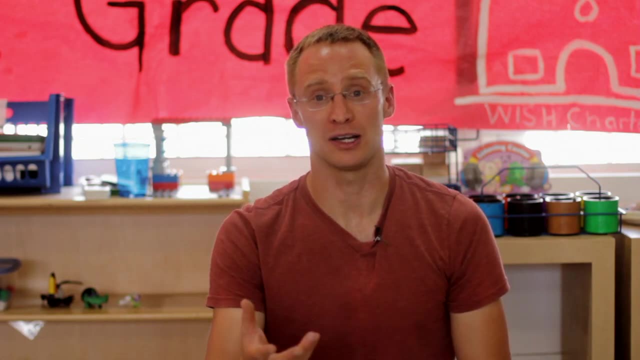 dumped in there And you can make it easier or harder. Maybe the first time you do it you just do two numbers, Put in two and three Dump And then, as the year goes on, you've got to change up the language and make it more sophisticated and work in the word plus. 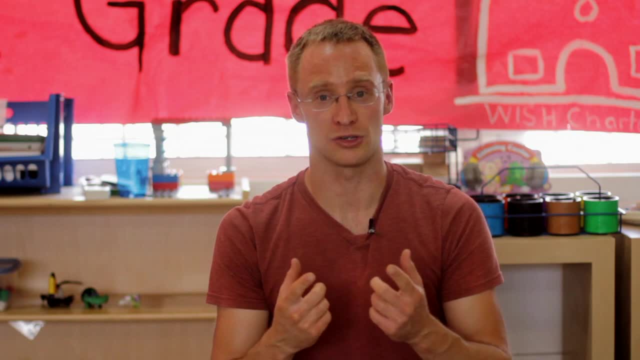 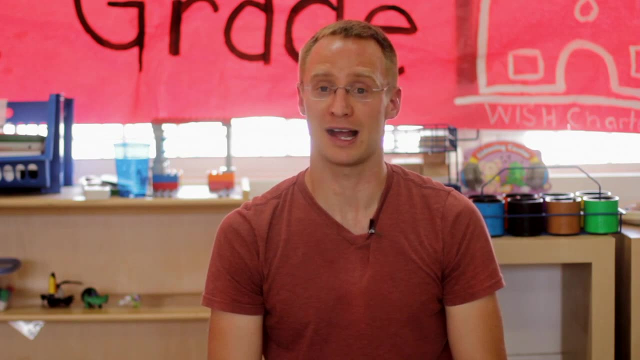 All along they're getting an idea that addition and the words that go with addition are about gaining, putting more in. This is Steve Rostowitz telling you a couple of activities you can do to develop math concepts in kindergarten. I'll see you next time.